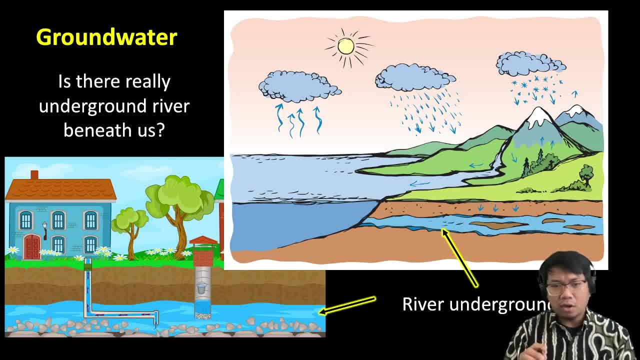 groundwater. there's always this misconception that I often find out there. For example, it often illustrates that there's a river flowing underground, as you can see here in this picture on the right side, as well as this picture right here on the left side, Right. so both picture shows that we have rivers. 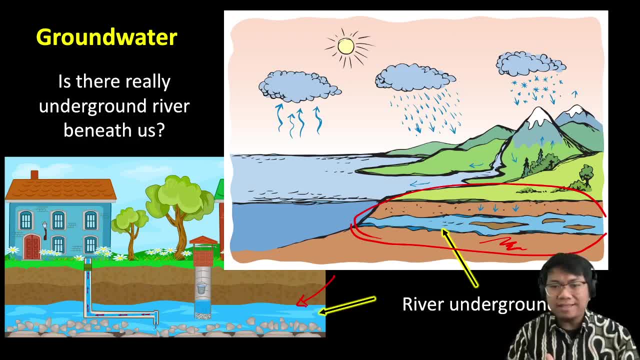 that flow underground, and in most cases, I have to say that this is not true. Alright, of course, in some cases, yes, this could be true, especially if you're dealing with limestone bedrock that can easily dissolve in water and eventually can create rivers underground, but in most cases, this is not true. that 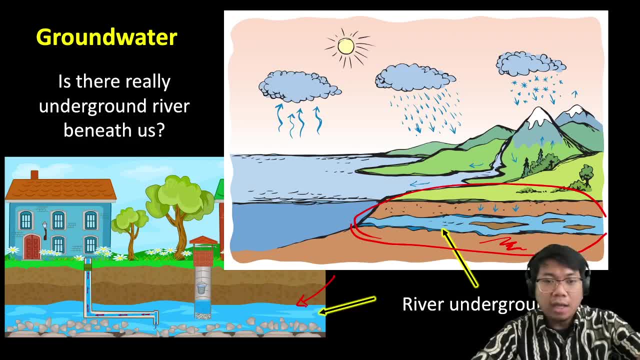 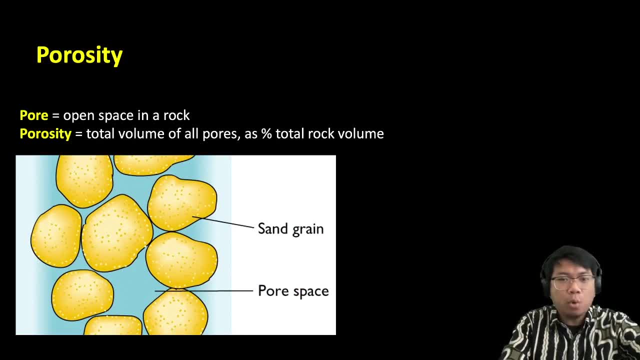 we do not have rivers underground, because water underground is often stored within what we call as pore spaces. okay for spaces. so what are pore spaces? again, pore spaces are just empty spaces that are located in between the grains of sediments. okay, so, for example, this could be a: 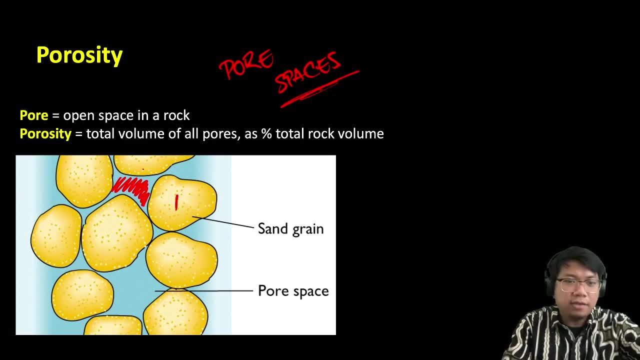 sandstone, and here i have one sand grain, two sand grain, three sand grain, four sand grains. right here we have four sand grains and in between those four sand grains we have the empty space in between, and this is what we call as a pore space. okay, pore spaces um, and rocks have this important. 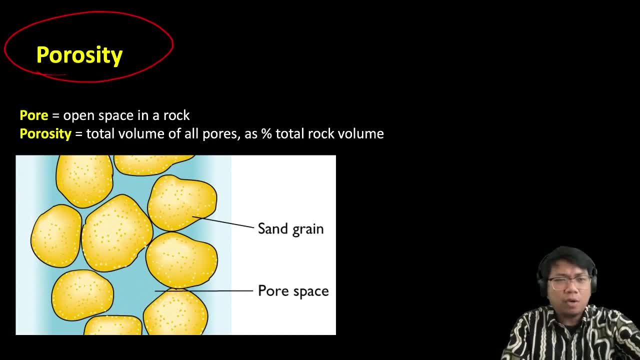 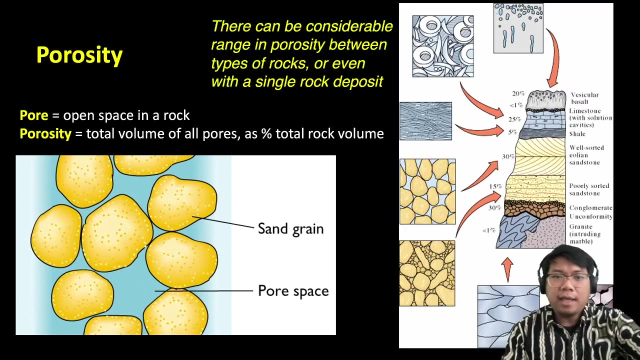 property which is called porosity. and what is and what porosity is, is that it is a total, the total volume of all pore spaces that is measured as a percentage of total rock volume. okay, all right, and there can be considerable range in porosity between different types of rocks, or 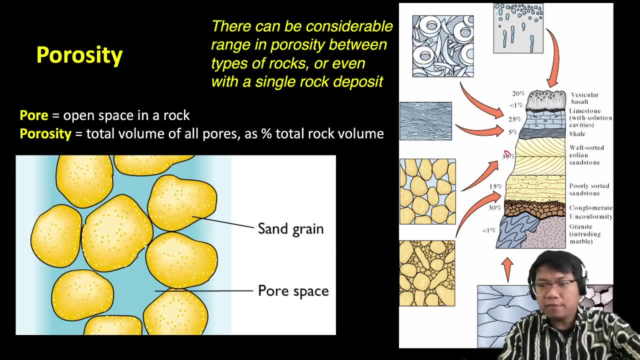 the same type of rocks, for example, here let me give you, let me highlight one of the best example for uh rocks that have high porosity, right, 30 percent for alien sandstone. so sandstone is a very is a type of rock that is very well known to have high uh porosity. okay, which? 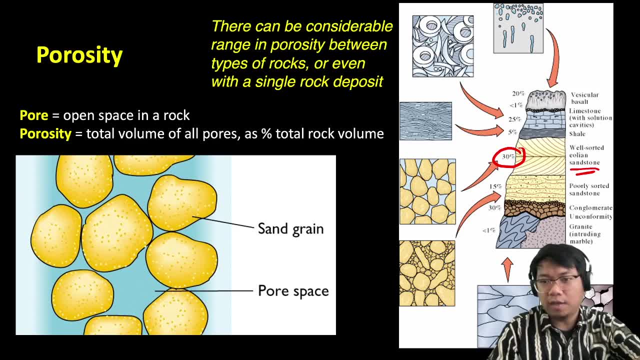 means it has lots of pore spaces within the rocks, okay, and we could also have some other types of rocks, for example like limestone, especially weathered limestone, or vesicular basalt- right here, all right, and some other rocks, for example, crystalline rocks, such as igneous rocks. 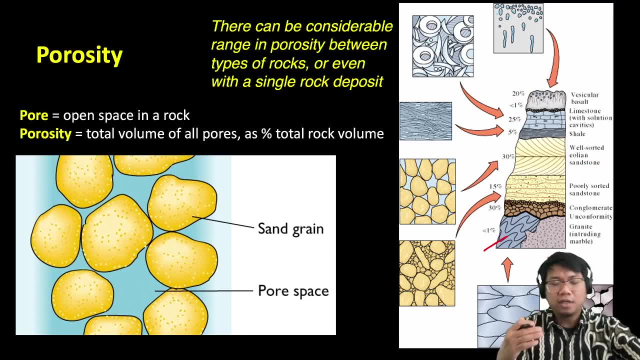 or metamorphic rocks. these are known for their porosity here, but this is a very common problem. these are rocks that have that, that commonly have a very, very low porosity, and in this example- look at this- it actually gives less than one percent of porosity, which means it's almost 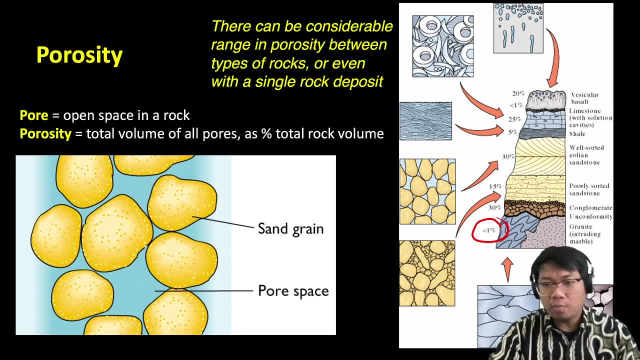 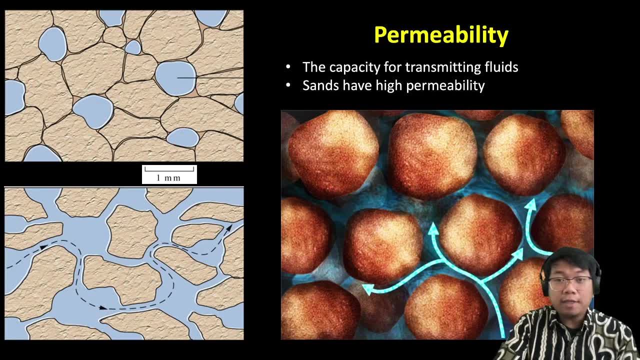 nothing right. there's almost virtually no porosity at all within the rocks. the second uh rock property that i would like to introduce you with is called permeability. so what is permeability? it is actually the ability for the rocks to transmit fluids, and in this case, of course, we're talking about groundwater. okay, so, for example, just to give: 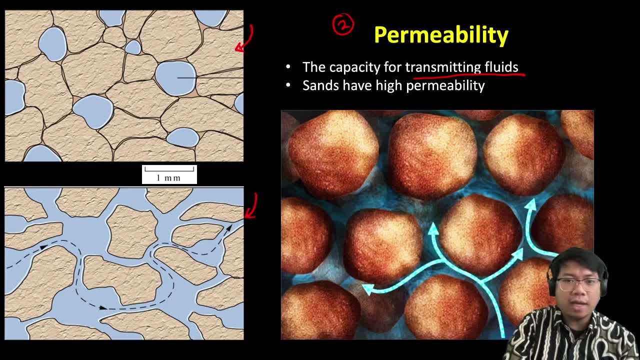 you a better illustration of this. i have two rocks: rock a at the top and rock b at the bottom. here, rock a has pore spaces illustrated by these blue areas right here. okay, so we see some pore spaces within rock a, and rock b has obviously has a lot more. 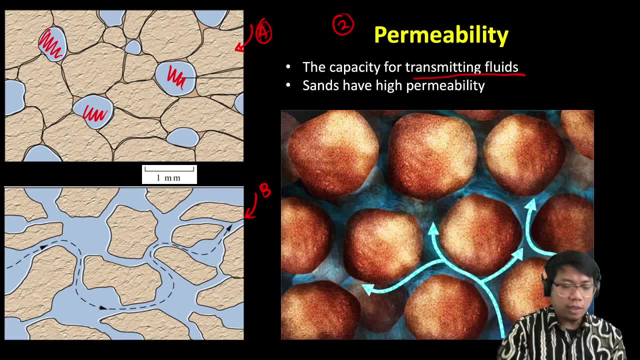 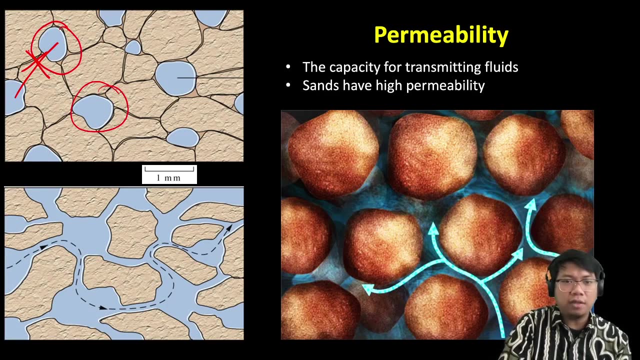 pore spaces, but one of the most important thing that we need to highlight here is that the pore spaces within rock a they are just not well connected. okay, for example, we have isolated pore spaces right there, another one isolated right there, another one isolated right there, so these pore spaces are not in communication with each other. 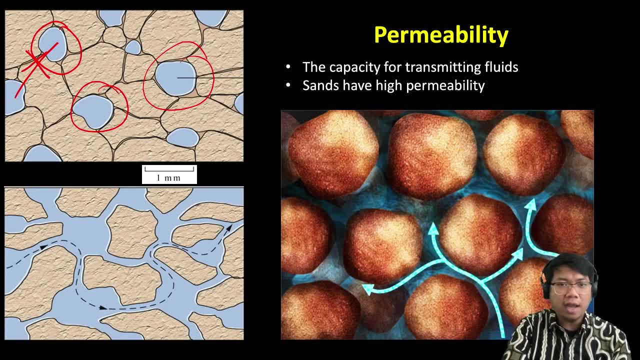 so therefore it can be considered. as you know, rock a has a very low permeability, okay, whereas rock b- here we see lots of blue areas, but again, the most important thing here is that those blue areas are well connected okay, and these well connected pore spaces will allow this rock to be able to transmit fluids easily, say from point a here on the left. 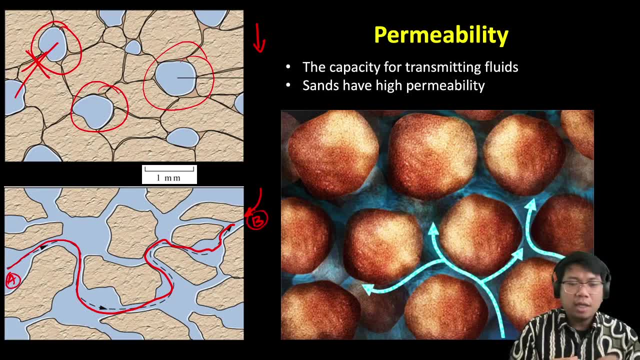 to point b here on the right side. so therefore, the permeability for rock b is much higher than rock a. okay, so those are the two main properties, rock properties, that i want you to know: porosity and permeability. okay, now, what are the type of rocks that have relatively high? 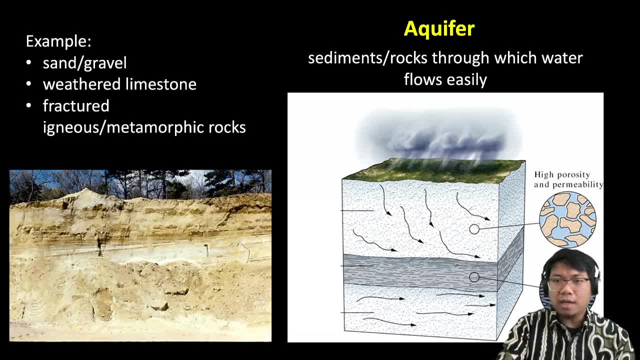 porosity and high permeability, and that rock is called aquifer. okay, so aquifer is a you know, sedimentary rocks or rocks that, um, that water can flow easily. okay, these rocks are typically known to be a very good rock, that that is able to hold lots of water as well as to allow the water to flow. 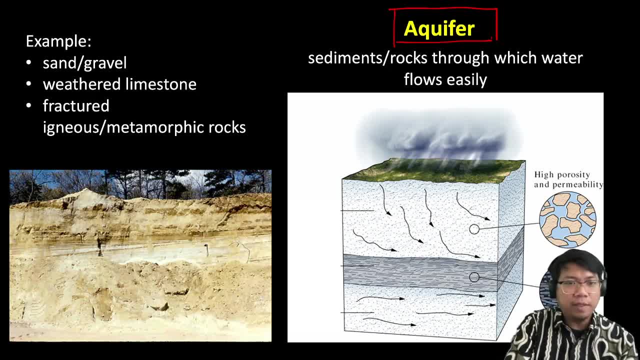 easily through it. okay, and the example for that would be sand and gravel, okay, weathered limestone, or we could also have some, uh, crystalline rocks, but it must be fractured. okay, these crystalline rocks must be fractured again to allow, um, you know, some openings within the rocks. 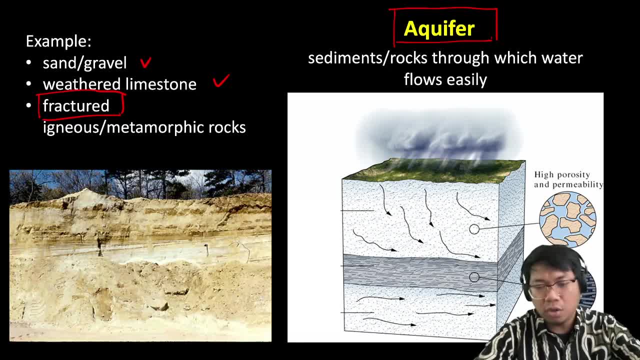 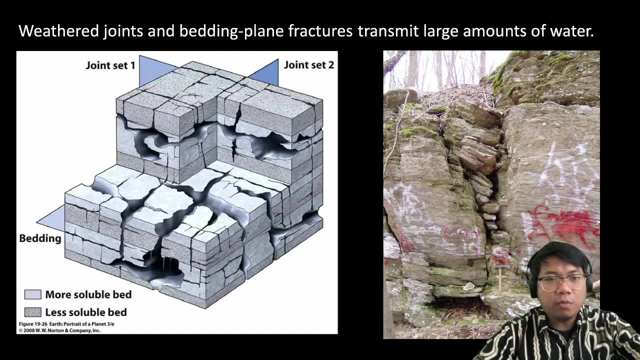 and allow the permit, you know the water to go through easily through it. okay, and here is an example of weathered joints and bedding plane fractures that can transmit large amounts of water. so this is what it looks like in nature right here. so even though, if you're, if we're having like crystalline rocks with- uh, you know, you know. 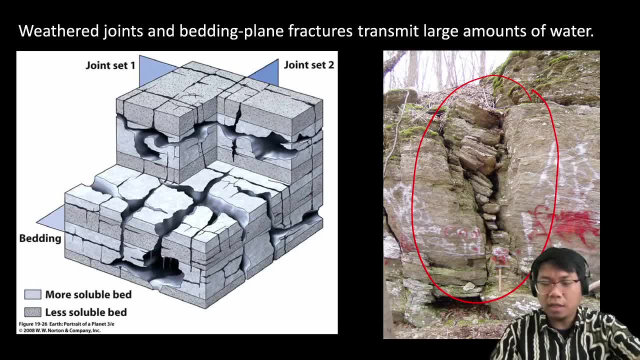 some very high porosity and permeability and some very low porosity and permeability. we're not going to be able to have a very high porosity and permeability as long as we have this fractures within rocks, and these are basically also open spaces within rocks that the water can occupy. 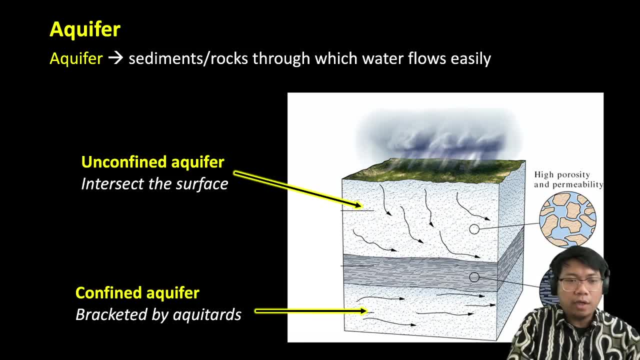 all right again. aquifer is a sediment rock through which water flows easily, and there are two types of aquifer that we know. the first one is called and confine aquifer and the second, unconfined aquifer, is- uh, this one right here, at the top of this picture, right here. 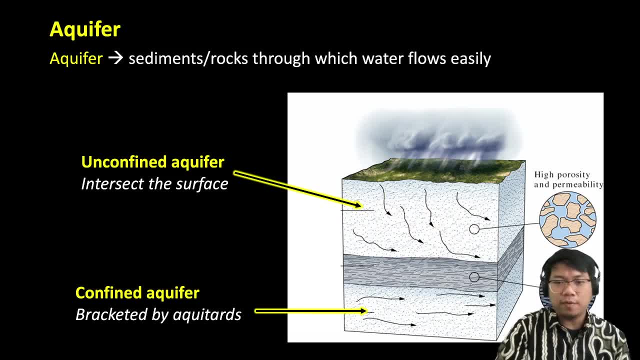 um, that the top of that aquifer intersects with the surface or the, you know, the ground surface. okay, so there's nothing holding right above that aquifer and that'll be called unconfined aquifer. now that is completely different with confined aquifer, of course, confined aquifer typically is. 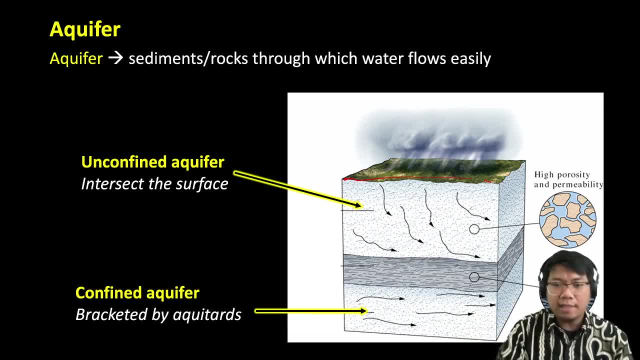 kept by what we call as impermeable layer right here. okay, so we have con. we have an aquifer here and at the top of it there is impermeable layer that sits on top of that aquifer and that will be called unconfined. 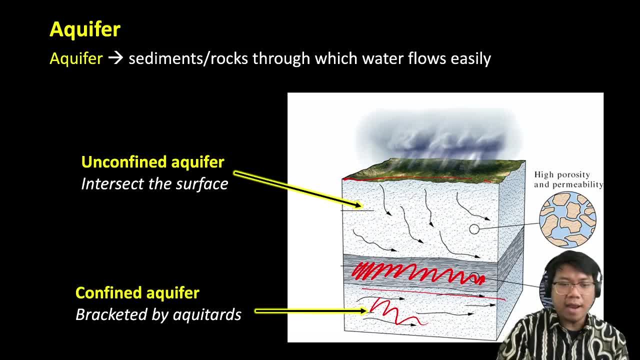 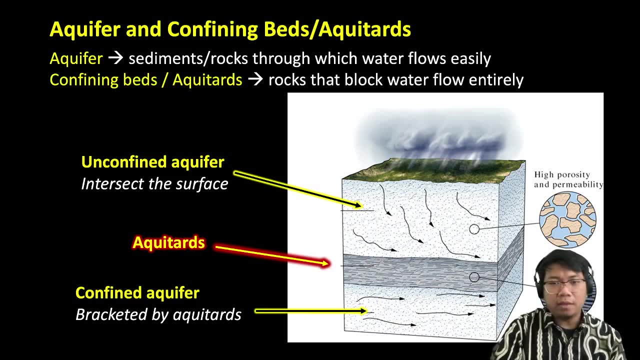 aquifer. okay, what is this? it's bracketed by aquitard. so what is aquitard? aquitard are rocks that block water. um, that blocks water flow entirely. okay, and in this example, it is illustrated by this impermeable layer that sits right here in between the two aquifers. 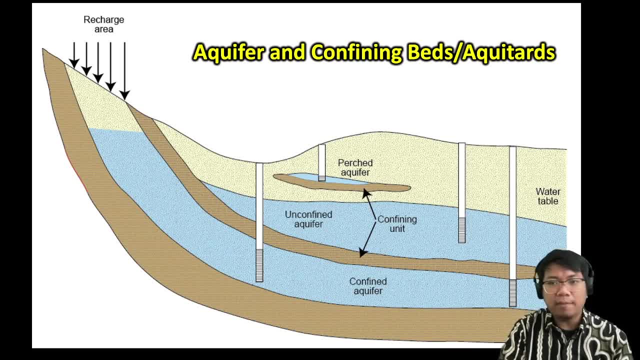 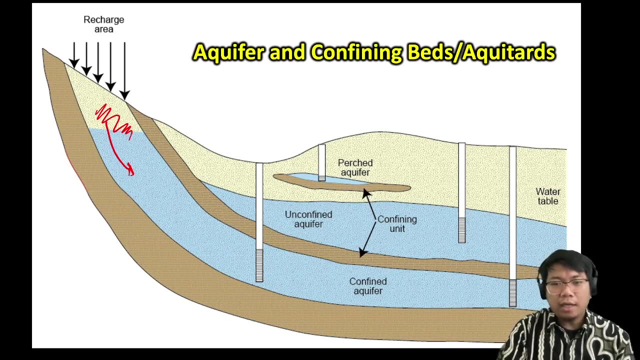 okay, so here's another example of aquifer and confining beds or aquitards. okay, so aquifers are illustrated by this yellow area right here, as you can see, here it got filled with water and here we have unconfined aquifer sitting at the top. here again, the 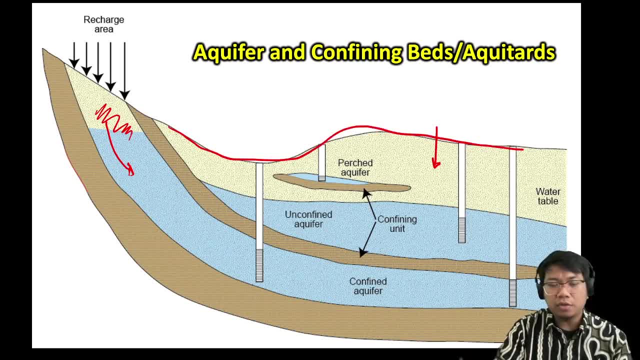 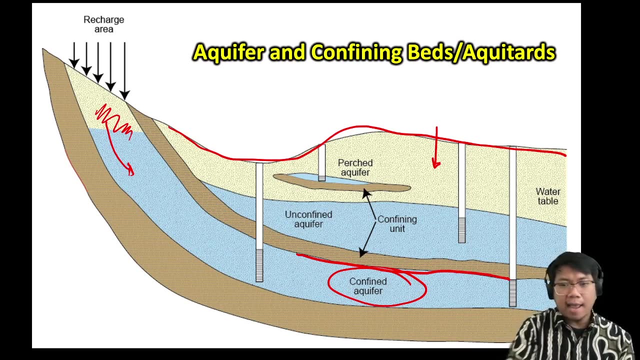 top of this aquifer intersects with the ground surface, whereas this one here is called confined aquifer, because the top of the aquifer is bounded by an impermeable layer or an aquitard. okay, now one might ask: okay, um, if we have confined aquifer that has impermeable layer? 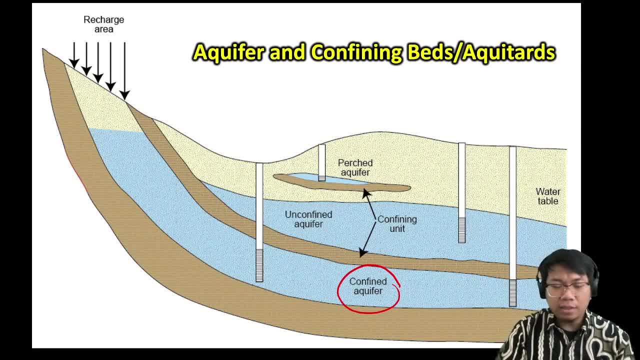 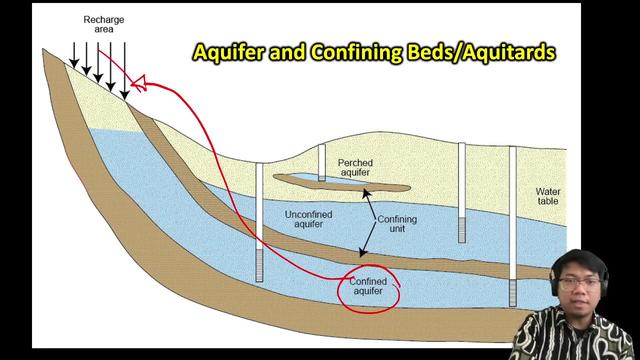 at the top of it. how do we get water into that confined aquifer? and the answer for that is that the though for the dual characteristics that we have in the��ic Europeans and all of that is that is the recharge area for that aquifer- is actually way. 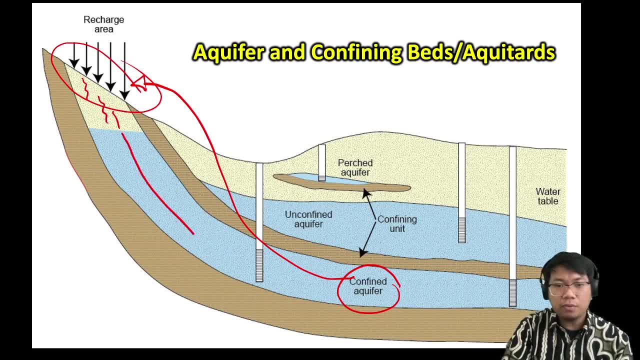 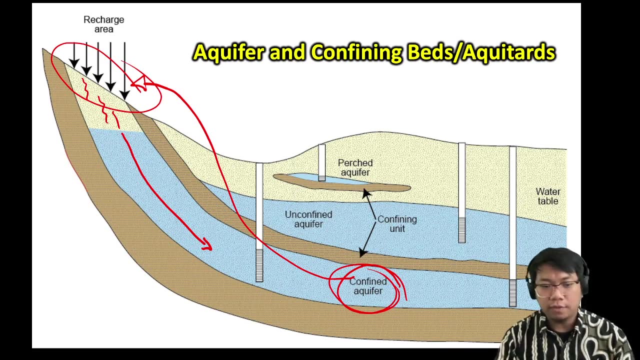 upstream of that aquifer. typically it happens, the recharge process happens in higher elevations, allowing the water to seeps into the ground, all right, and flows downward and fill the confined the stuff that i would like you to know for this, uh, for in this video, okay, and i'll see you again.